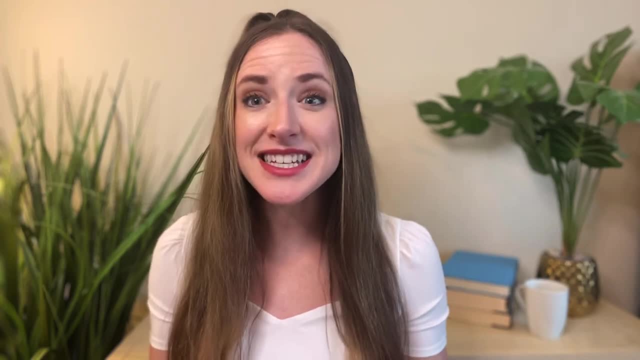 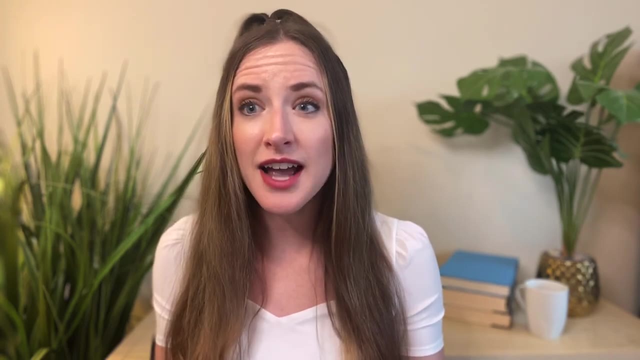 a unique symbol to represent it, For example, the click sounds that you make with your tongue. the IPA has symbols for those. The Sid the Sloth's iconic Sid the Sloth sound for the movie Ice Age. Doesn't anyone love me? Isn't there anyone who cares about Sid the Sloth? 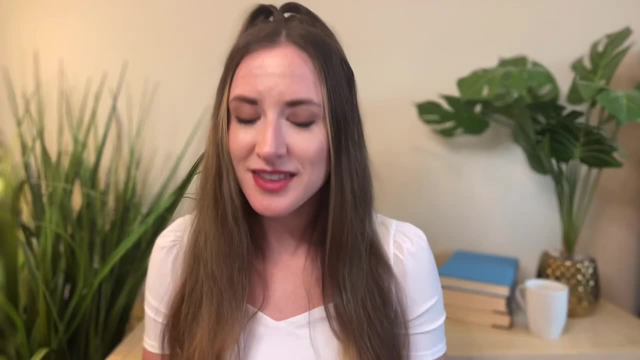 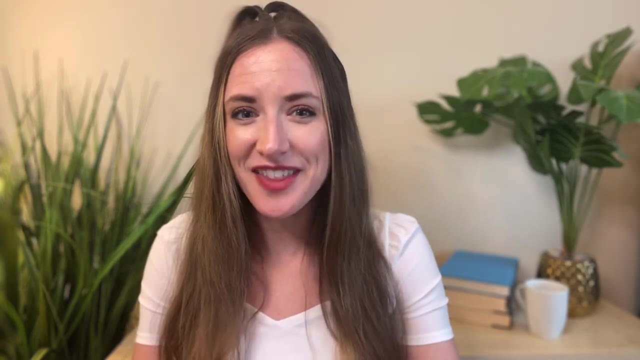 The IPA has got a symbol for that. And the sound you make to imitate a lawnmower: Yeah, the IPA has a symbol for that too And, fun fact, even though we don't use those sounds in English, they're all real sounds. 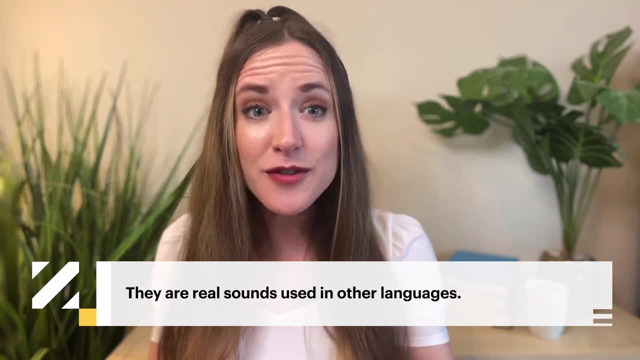 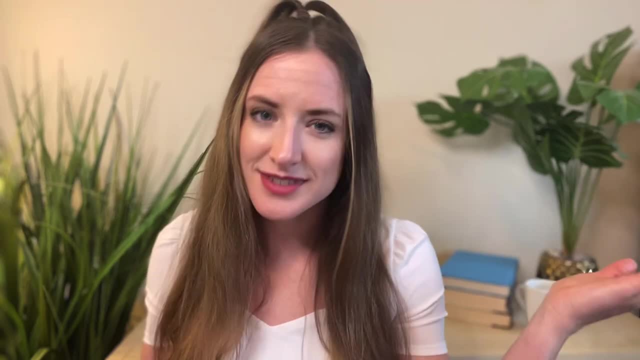 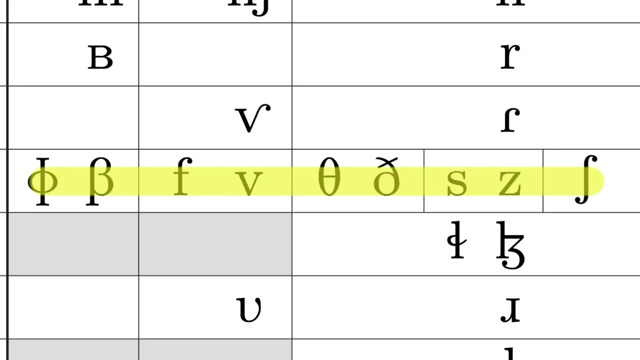 used in phonetic systems in other languages. Clicks, for example, are very common in African languages, The sound is used in Icelandic, And the- which is my personal favorite- is used in several languages spoken in Papua New Guinea. Now, the IPA doesn't just provide us with symbols to represent all of these sounds, It also 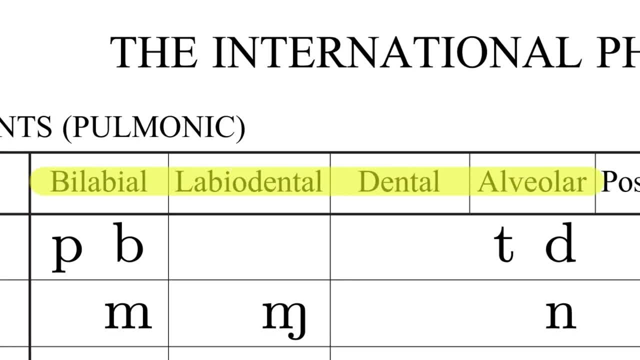 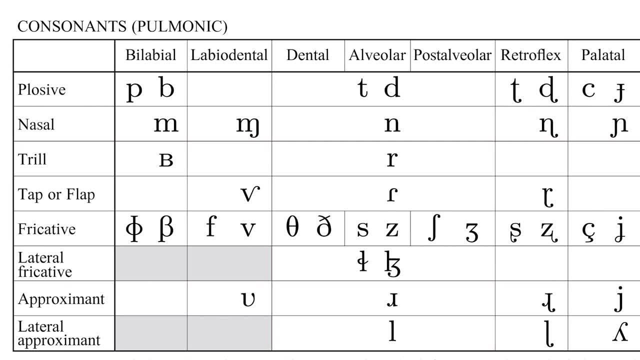 provides us with clear descriptive and technical terms by which we can describe them. For example, the technical term for my personal favorite sound, the, is a voiced bilabial trill, And by the end of this video, you'll have a much clearer understanding of how IPA symbols. 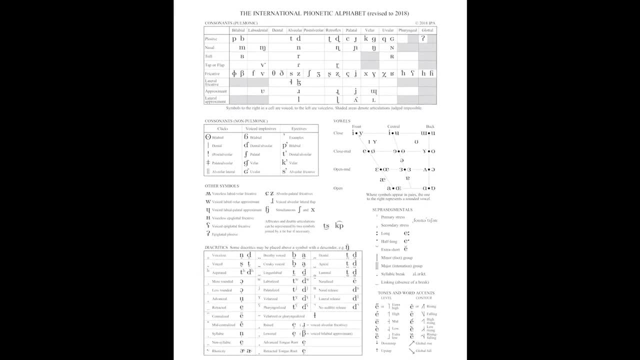 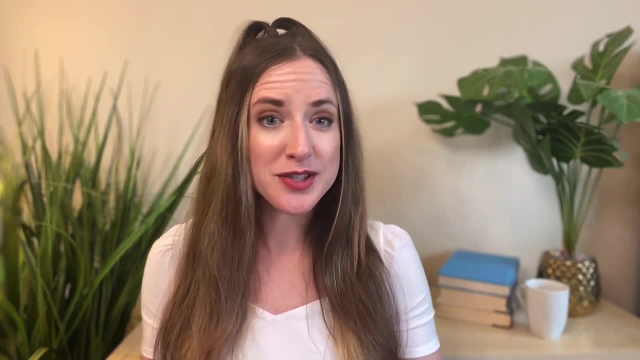 get their technical names Now. the IPA is obviously a very helpful tool for trained phoneticians, but it's also quite useful for any curious mind who wants to be able to read the phonetic transcriptions in dictionary entries, or for language learners who want to better understand how to make. 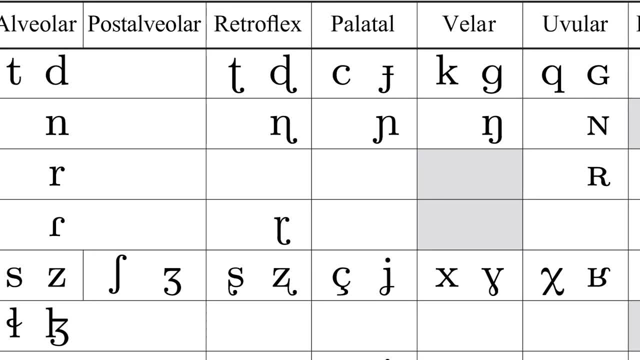 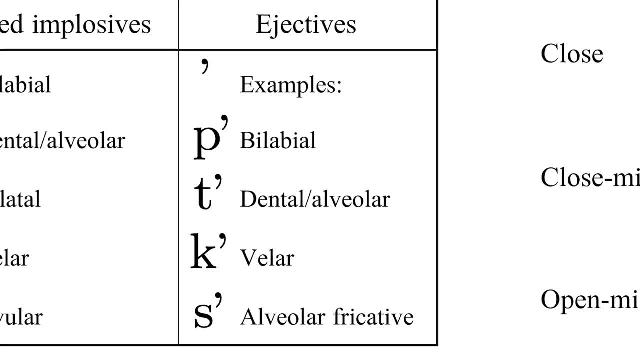 specific sounds in their target language. And here's some really good news: If you already know written English, you're already halfway there to understanding IPA. That's because, while the IPA does rely on a lot of Greek letters and other symbols that you might be unfamiliar with, 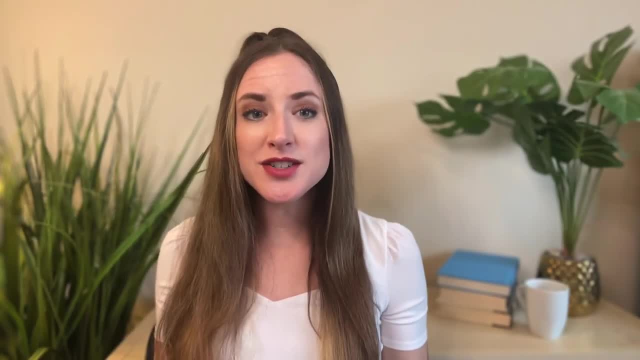 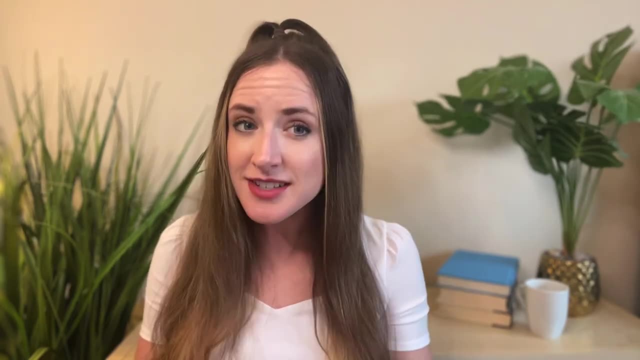 Use most of the letters from the English alphabet. So what do you need to know about the IPA in order to start reading and writing it? Well, like I said earlier, the IPA is one single sheet of paper, but there is a lot of information on it. So where should you start? Well, you should start with the consonant. 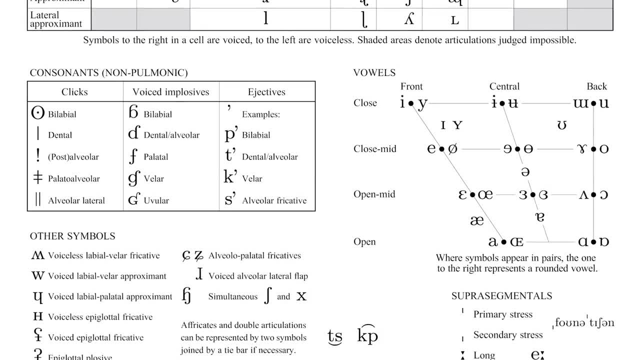 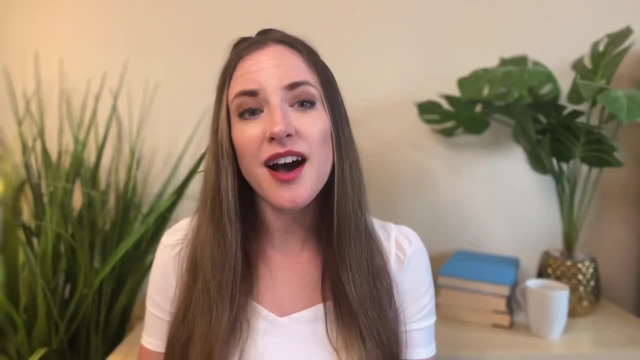 chart and the vowel map. Those are your keys to understanding the IPA. Everything else is just details. Consonants are sounds like b, d, g, c and vowels are sounds like a, e, o, u. Now let's. 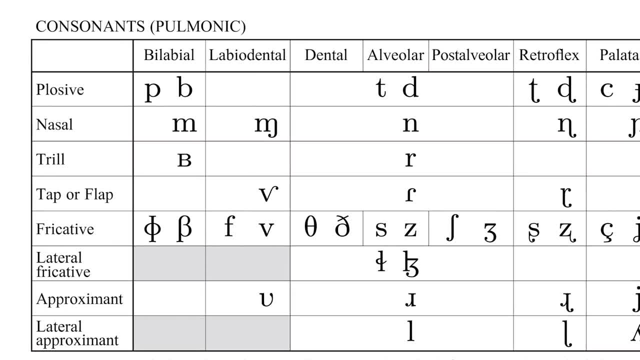 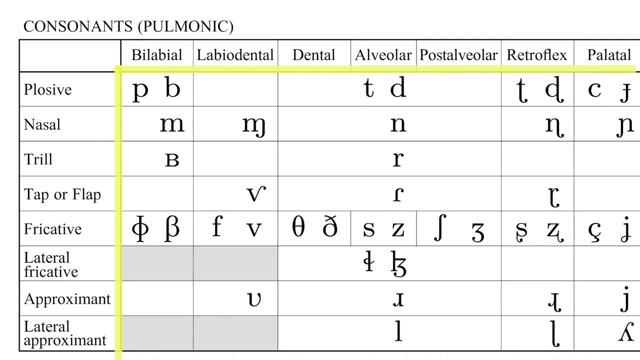 start with the consonant chart. The consonant chart is simply a table made up of a bunch of columns. in rows. The columns are organized by something called the place of articulation, which really just means where, in your mouth, touching needs to happen in order to make the sound, So as you move from. 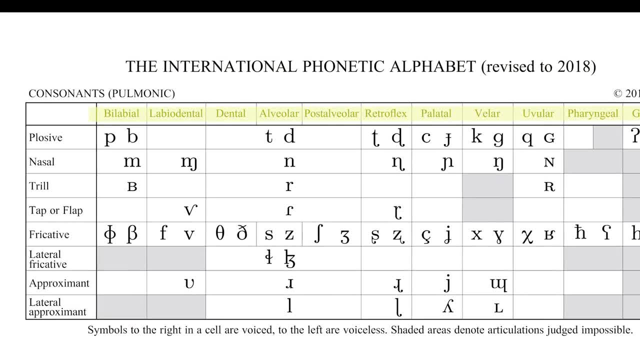 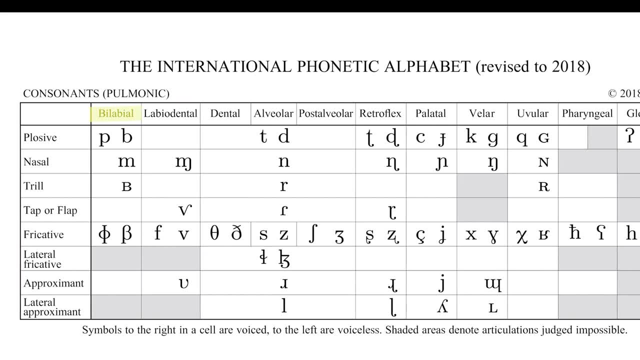 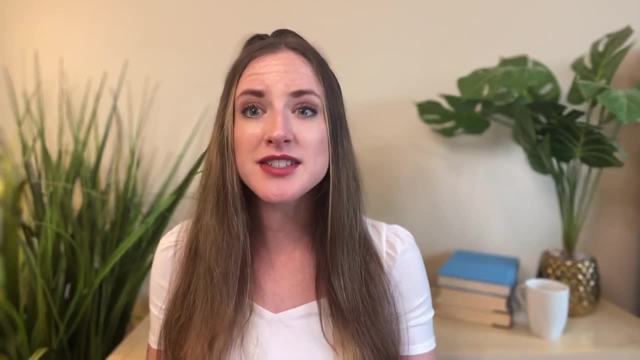 left to right on the consonant chart. the place of articulation within your mouth moves from the front to the back. For example, the leftmost column is called bilabial, So that column contains all the bilabial consonants. Bilabial literally means two lips, So this requires touching at the very front of your 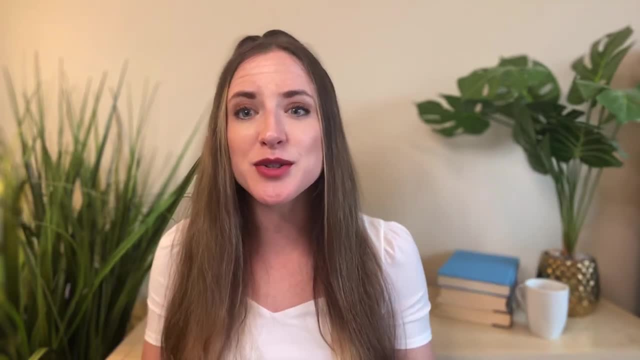 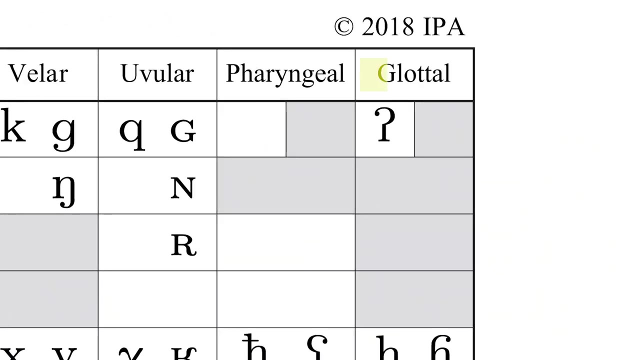 mouth. Some consonants in the bilabial column include b, p, m and my favorite one, the b. Now all the way to the rightmost column, you'll see glottal sounds. The name comes from the epiglottis, which is one of your articulators way back in the back of your 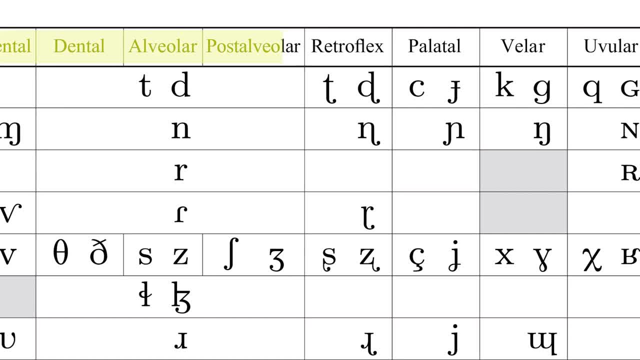 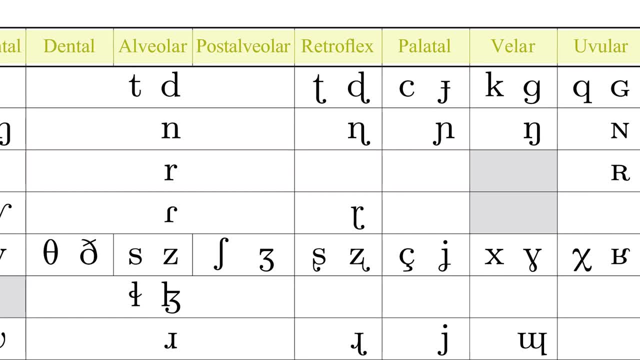 mouth, almost at your throat. As you can see, the names of the columns oftentimes give you a hint as to what, in your mouth, needs to be touching in order to make the sound happen. Ok, so the columns tell you the place of articulation. What do the rows tell you? Well, the rows. 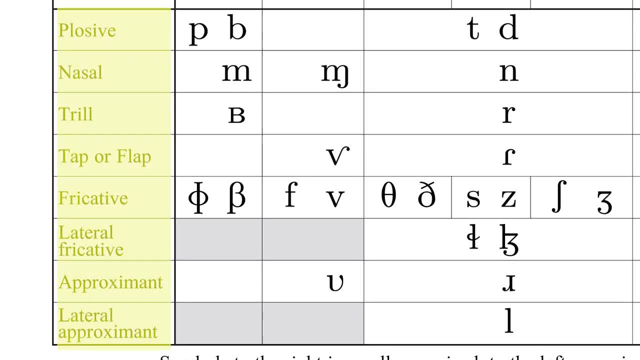 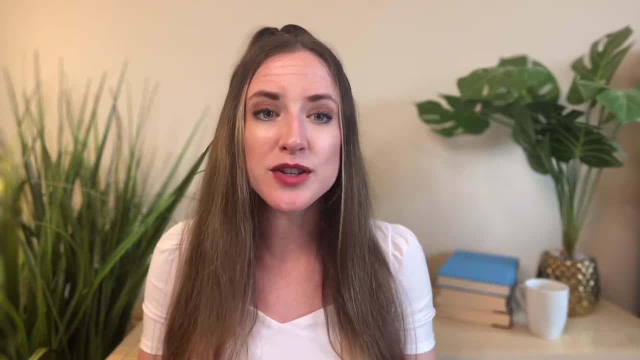 tell you the manner of articulation for the consonant. The manner of articulation has to do with the manner in which your articulators in your mouth move to modify airflow in your vocal tract. For example, the first row is labeled plosives. Plosives include sounds. 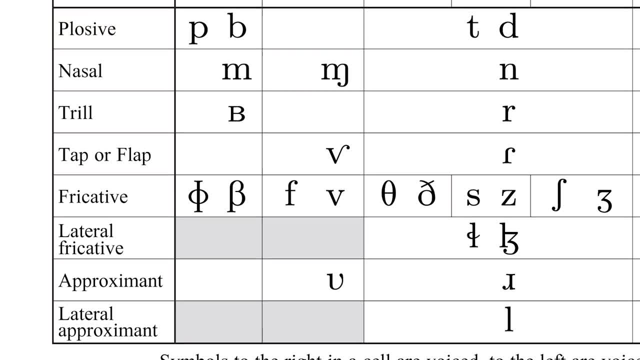 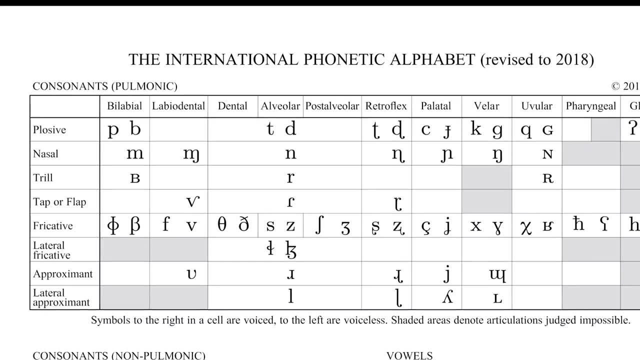 like p, t, k, b, d, g and are sounds that start with your mouth closed and then end with a burst of airflow being released all at once. if we go down a few rows, you'll see a row for trills. trills are the sounds like the spanish. 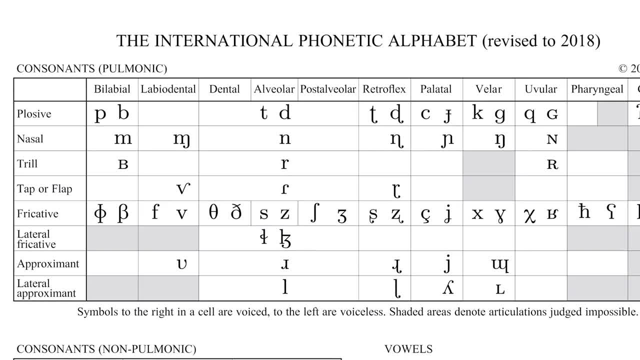 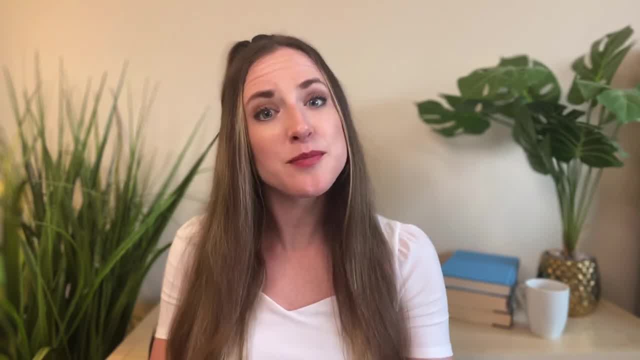 or my favorite lawnmower sound, that where a repetitive sound happens in quick succession. so now we know that the column that a consonant is in tells us its place of articulation and the row that it's in tells us its manner of articulation. there's one thing left if we think. 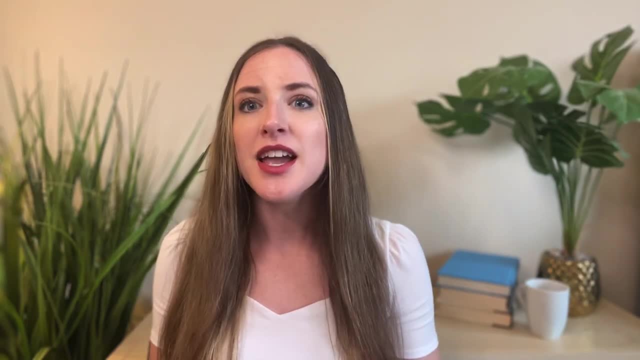 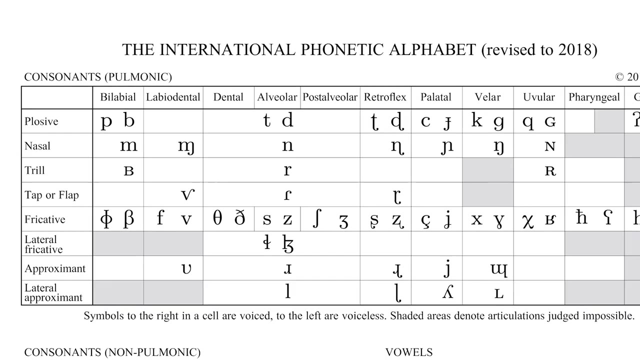 back to my favorite sound, the voiced bilabial trill. you know that bilabial refers to the place of articulation, meaning both lips touching, and the trill refers to the manner of articulation, so the lips touching multiple times in quick succession. but what does that word voiced mean? 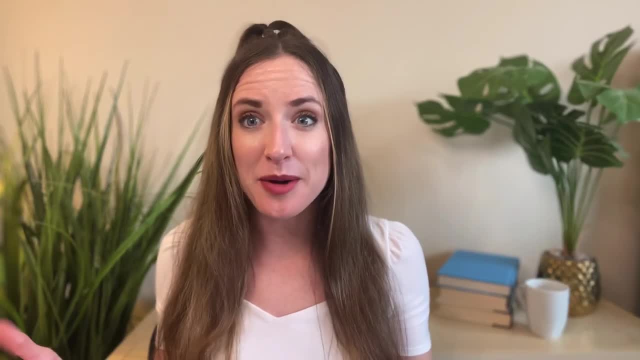 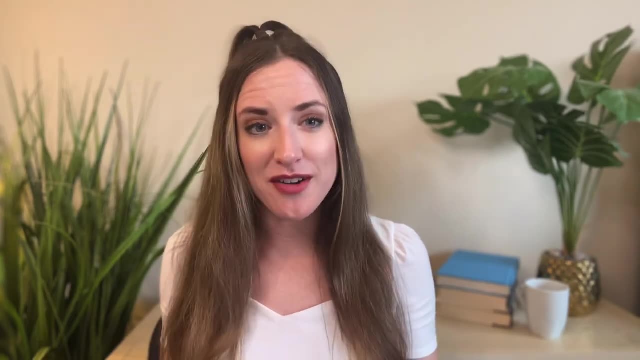 well, it has to do with your vocal cords, basically whether or not they're vibrating. if your consonant is voiced, that means your vocal cords are vibrating. if the constant is voiceless, they're not vibrating, and you can actually test this out right now by touching your throat, as you say. 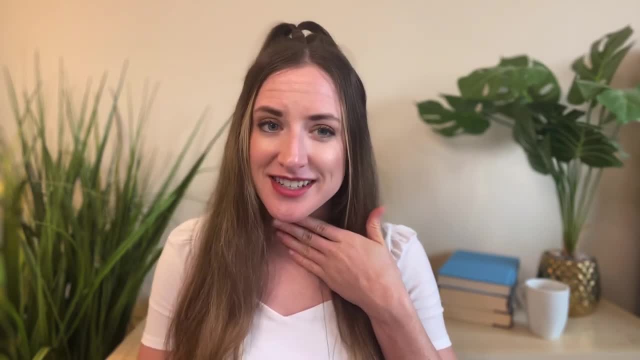 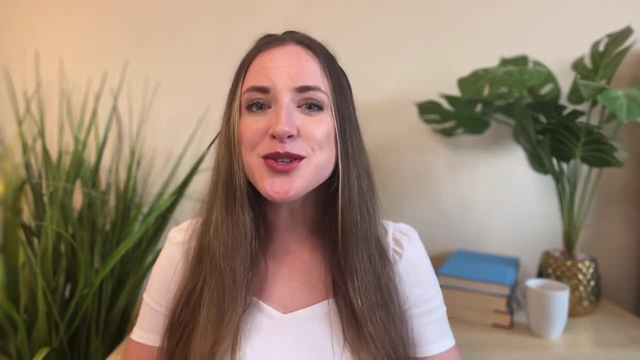 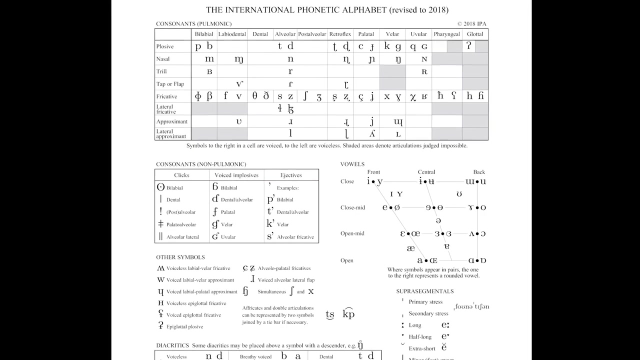 which is a voiced consonant and which is a voiceless consonant. see, now you know how the voiced bilabial trill gets its technical name and, more importantly, you also now have everything you need to start exploring the consonant chart on your own. but before you do that, let's talk vowels. that means we're headed. 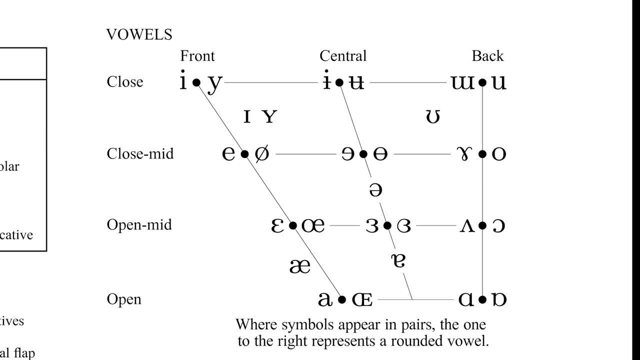 over to the vowel map. now there's a lot of cool stuff to know about vowels, but we're just going to go over the basics. the main thing that you should take away is that the vowel map is organized by the location of your tongue in your mouth. 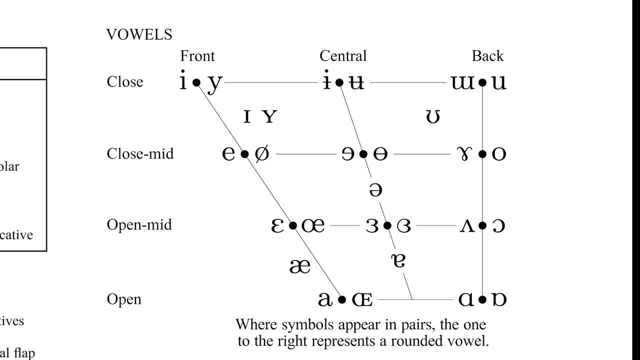 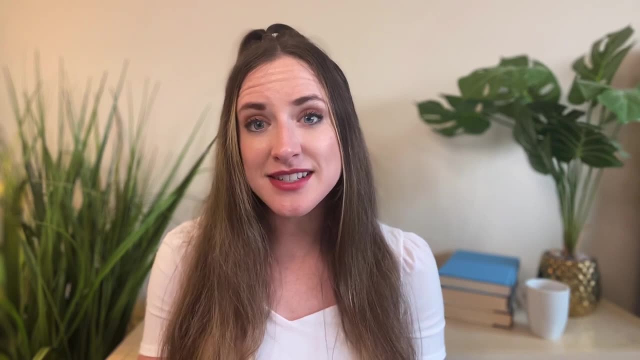 for example, the higher a vowel is on the vowel map, the higher your tongue needs to be in your mouth to make that vowel sound. high vowels like e and u require the tongue to be higher in the mouth than, say, low vowels like eh and ah, and the further to the right the vowel is on the map. 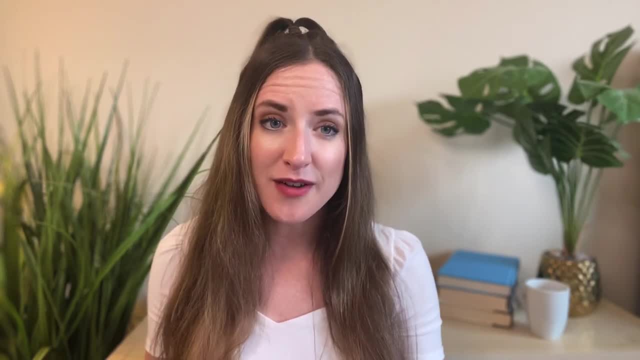 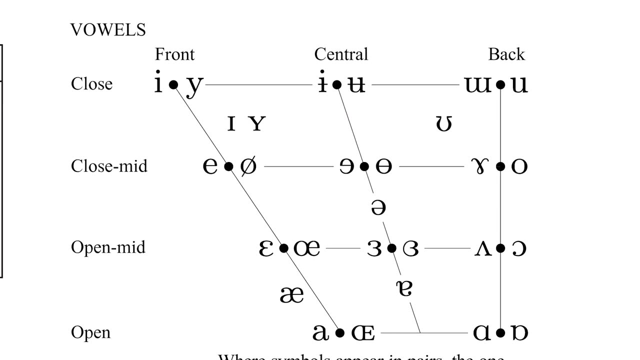 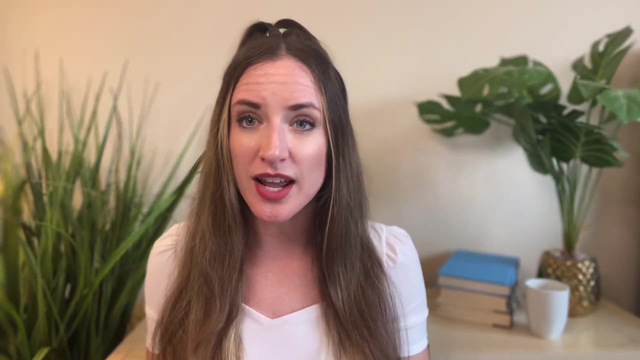 the further back horizontally your tongue needs to be in your mouth to produce that vowel sound. for example, vowels on the left side of the vowel map, like e and a, require the tongue to be further at the front of your mouth compared to vowels on the right side, like u and o. now you probably already know this, but it's worth mentioning. 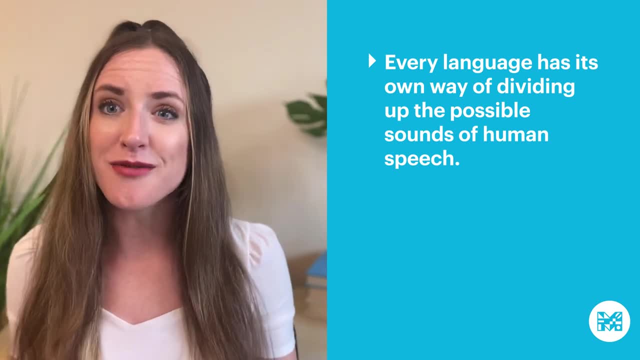 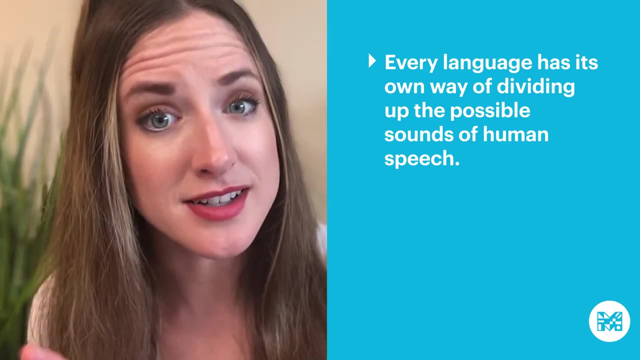 not all languages have the same organization or even number of vowels in their vowel systems. that's because every language has its own way of dividing up the possible sounds of human speech. this goes for consonants as well as vowels. well, my friends, there you have it, from clicks to trills. 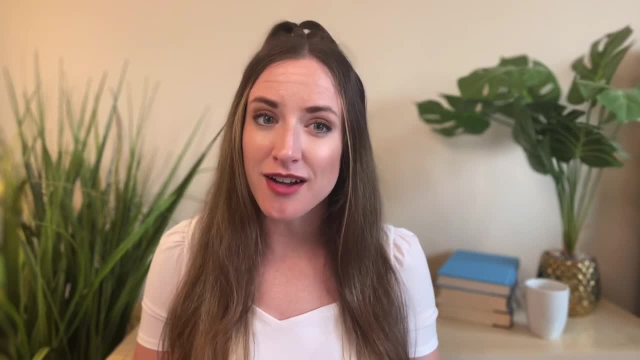 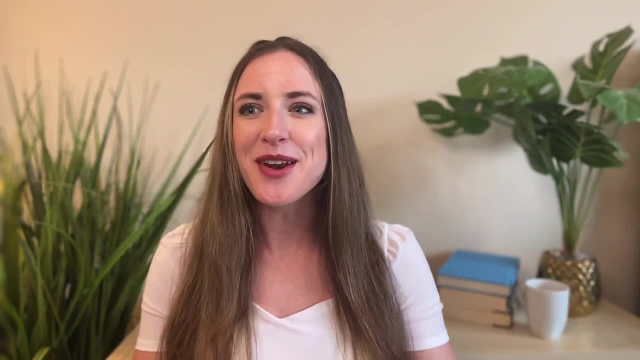 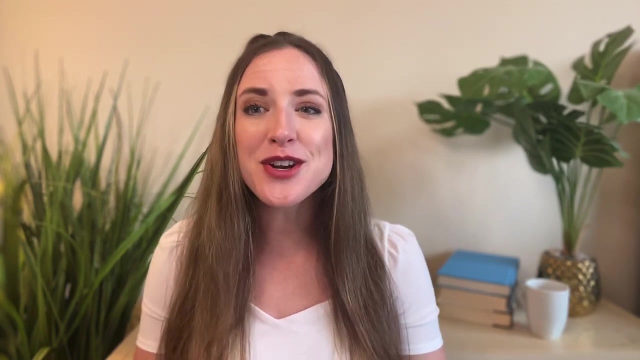 consonant charts to vowel maps. we covered a lot of ground in this video. the main takeaway you should keep in mind is that every language has its own way of dividing up the possible sounds of human speech. the ipa is a very special piece of paper that, with just a little studying, you can use to unlock the